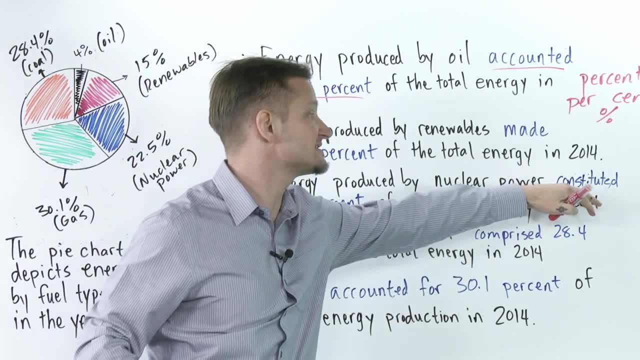 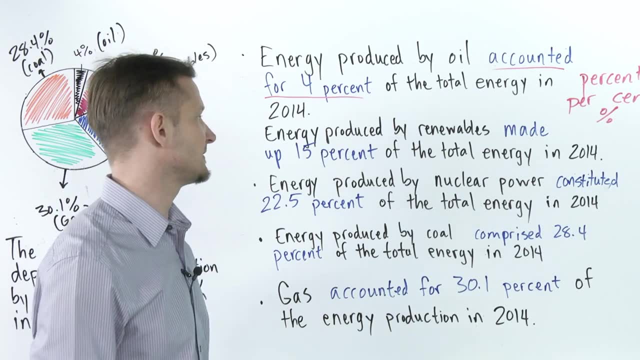 Next one: Energy produced by nuclear power constituted 22.5% of the total energy in 2014.. Two more of the total energy in 2014.. That's constituted 22.5%. Same thing, You can plug in any of these. 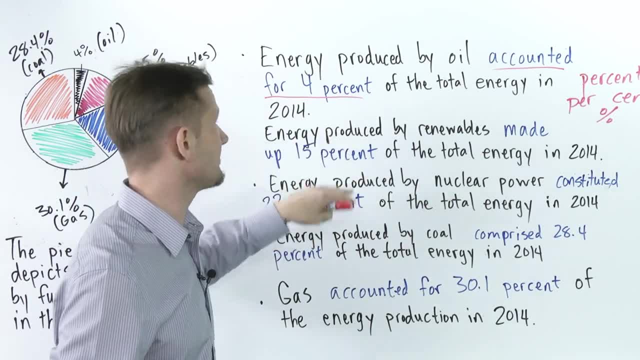 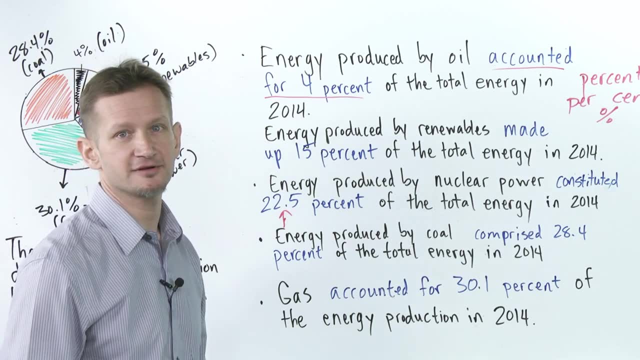 numbers into these patterns Constituted, made up, accounted for. Now here's something that you might want to look out: This dot right. Some people say 22.5.. Whatever you do, don't say 22.5.. 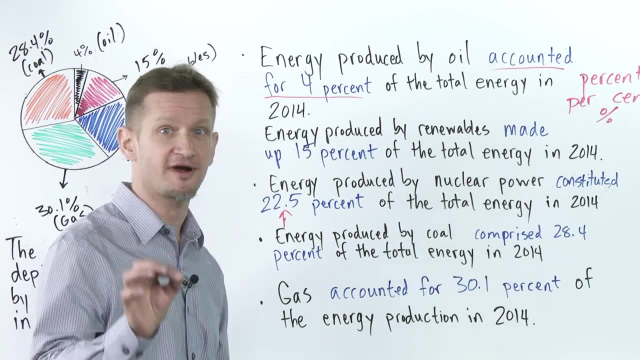 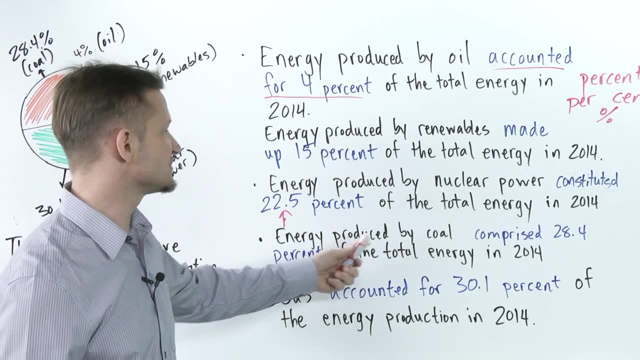 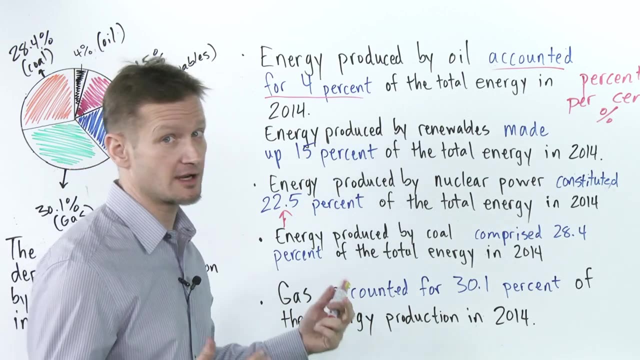 22.5.. Okay, 0.5, 0.7, 0.6, 0.whatever, All right. next, Energy produced by coal comprised 28.4% of the total energy in 2014.. Again, same thing You can use, comprised up here: Energy. produced by oil comprised 4% of the total energy in 2014.. You can swap them around, no problem. Last one, Gas, accounted for 30.1% of the energy production in 2014.. So yeah, as you notice, this is the same. 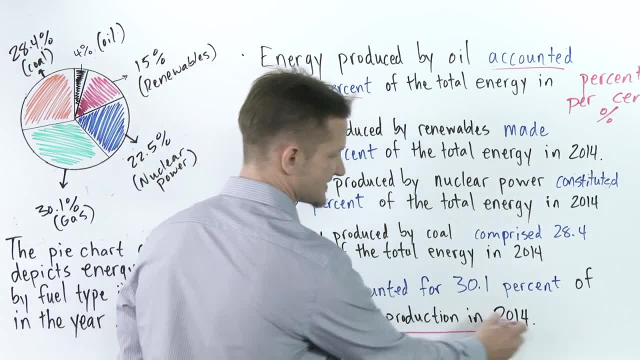 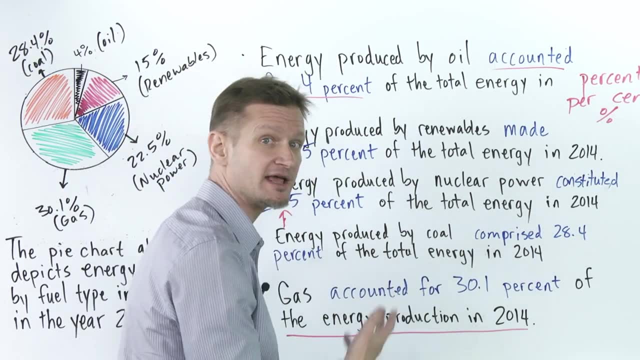 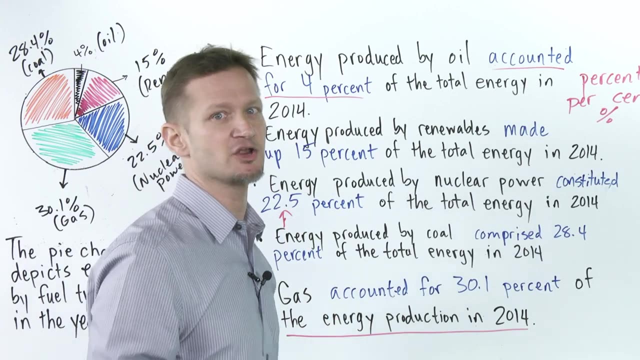 pattern up here, but we're just showing that you can change what comes after it, right? You don't have to just say the total energy in 2014.. There's ways that you can vary what comes after it as well, And that diversification of your vocabulary is going to demonstrate your ability to use the. 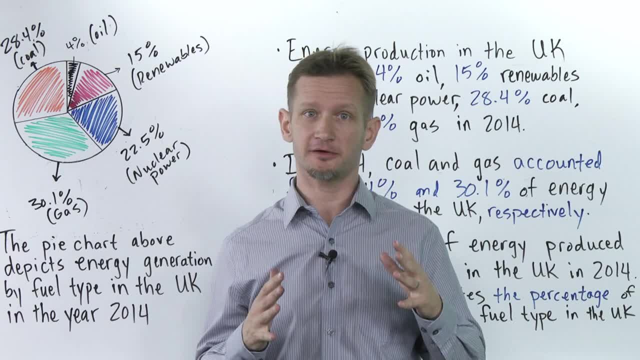 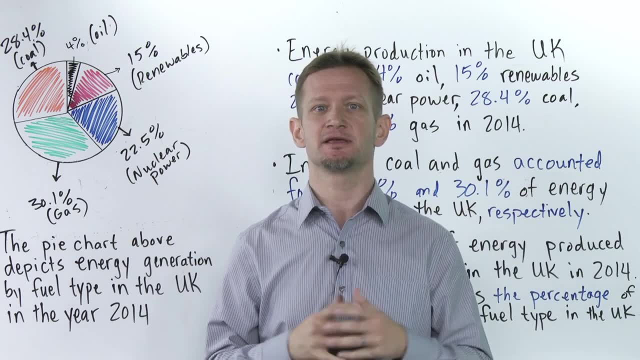 English language. Okay, so let's move on. We're going to talk about how do you compare two percentages, or talk about two percentages in one sentence. Let's look at a couple sentence patterns, Okay, so first off, let's look. 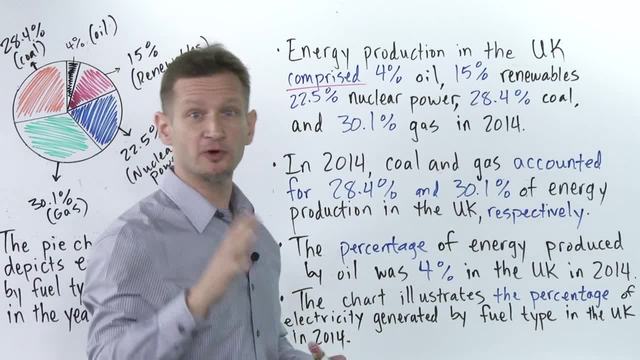 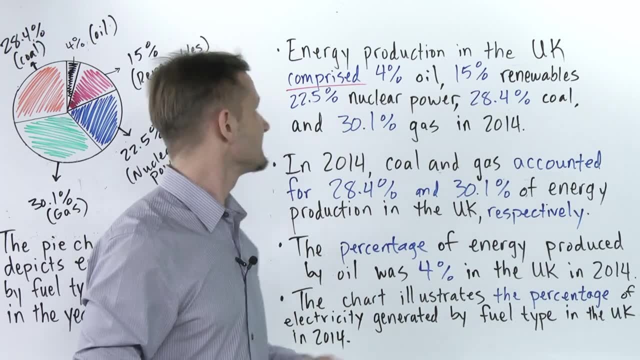 at this word comprised. Comprised is a really high level of vocabulary word. If you can find an appropriate place to use it and you can use it correctly, do it. Comprised means to be made up of, so energy production in the UK comprised and use it like a copy, But I'm not. 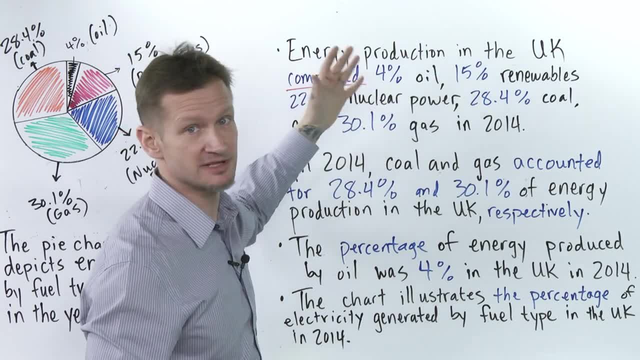 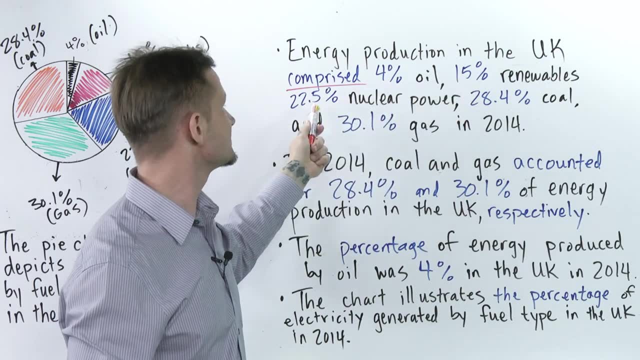 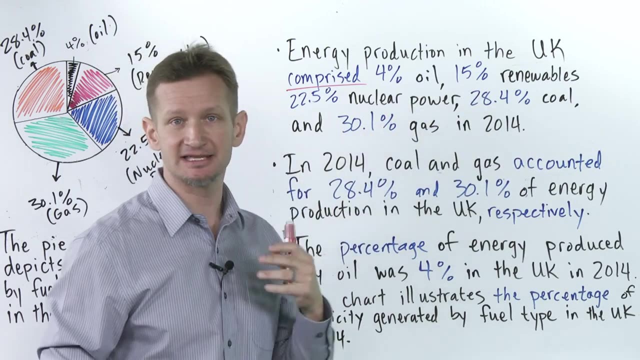 energy production in the UK is made up of means the same thing. Energy production in the UK comprised 4% oil, 15% renewables, 22.5% nuclear power, 28.4% coal and 30.1% gas in 2014.. So I 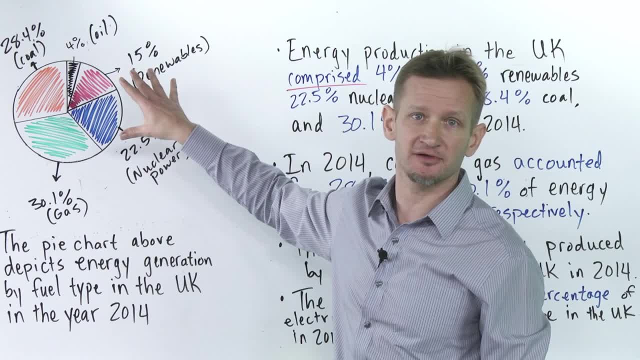 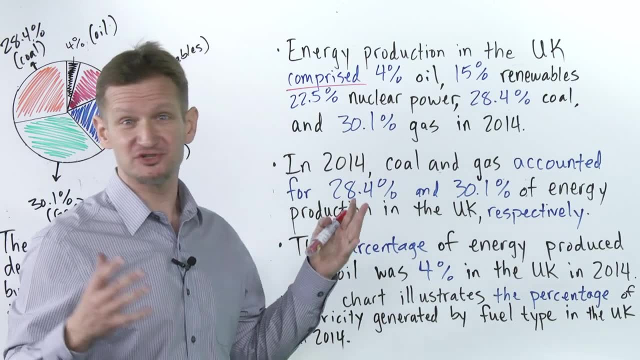 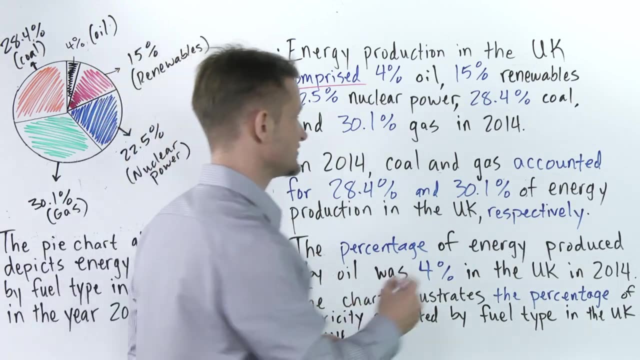 just did in one sentence, I described the entire chart in a really concise way. Okay, now perhaps you just want to talk about two percentages in one sentence, or maybe three, So there's a special word that you can use to do that, and that's called that's respectively: So in 2014, coal and gas. 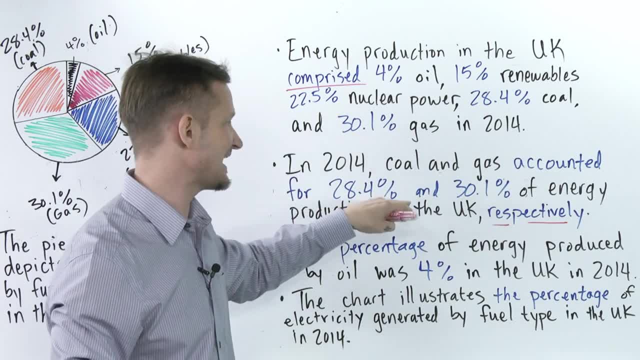 accounted for 28.4% and 30.1%. So in 2014, coal and gas accounted for 28.4% and 30.1%. So, in 2014, coal and gas accounted for 28.4% and 30.1%. 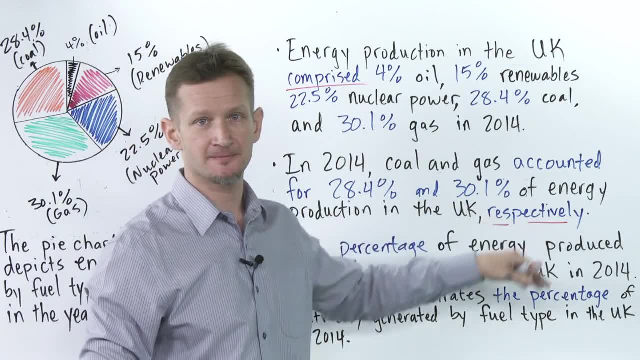 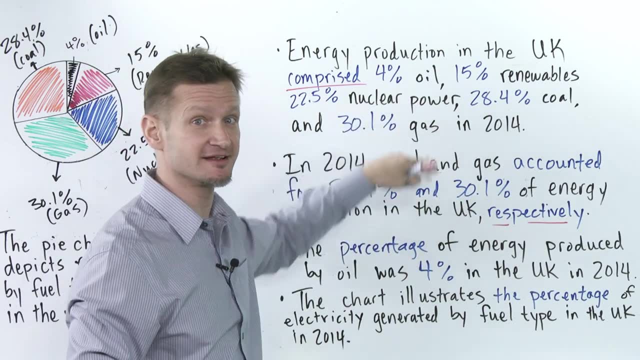 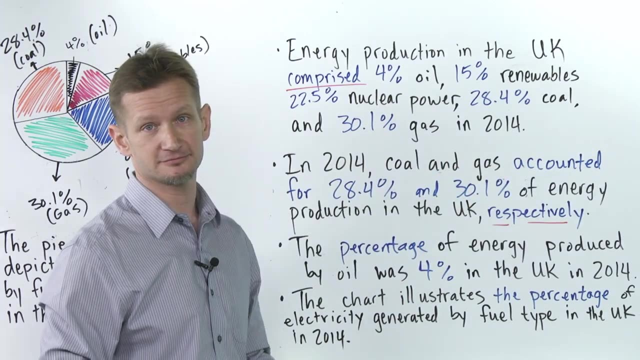 of energy production in the UK respectively. So this respectively means that these two numbers account for the two nouns that preceded it. So it went coal and gas, and so that means coal is 28.4% and gas is 30.1%. Okay, so respectively allows you to talk about two distinct percentages in one. 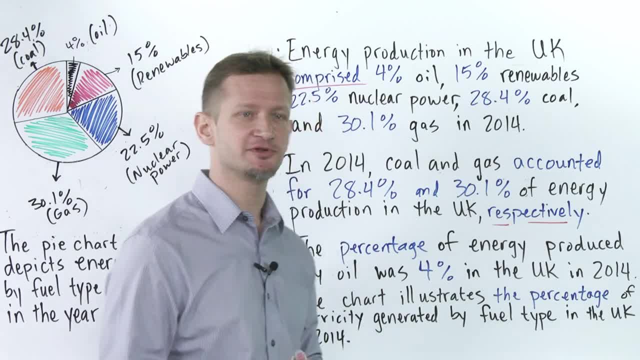 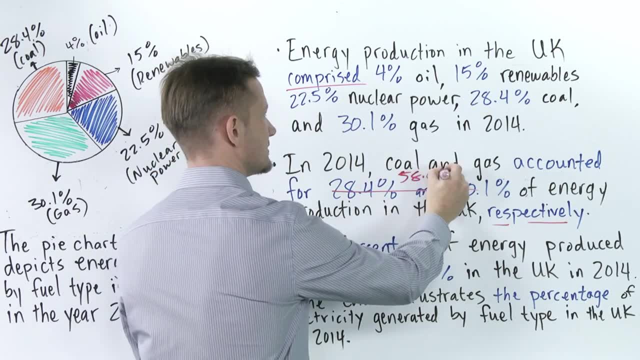 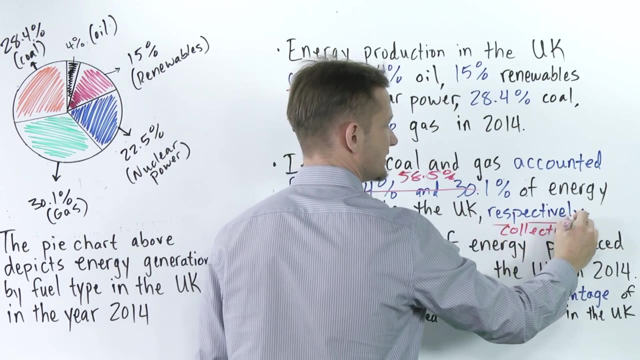 sentence. But what if you wanted to combine them? Well, this is how you would do that: You'd combine these two numbers And that is what is that? 58.5%? and then here you change respect Actively, you would change that to collectively right in 2014.. 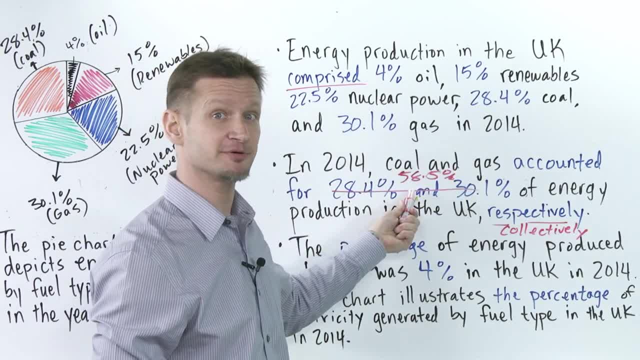 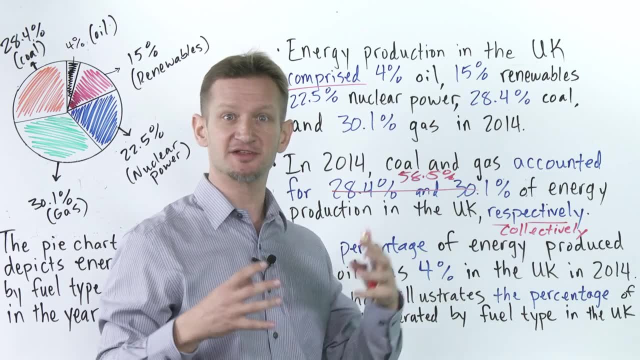 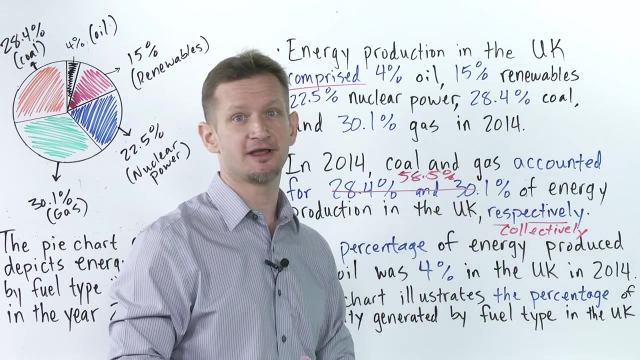 Coal and gas accounted for 58.5% of energy production in the UK collectively, and that collectively is just a way to let us know that those two percentages have been added together. So now you got a way to talk about them Separately and together, and if you can use that, that's going to help your score. 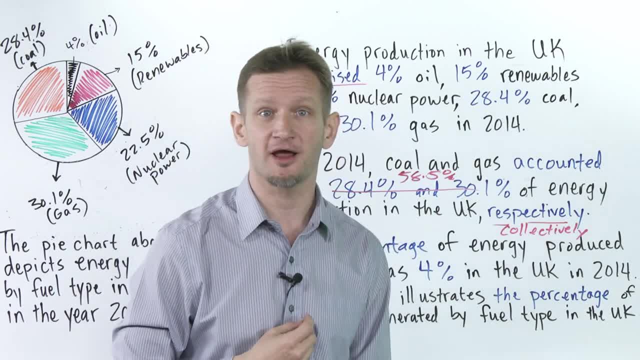 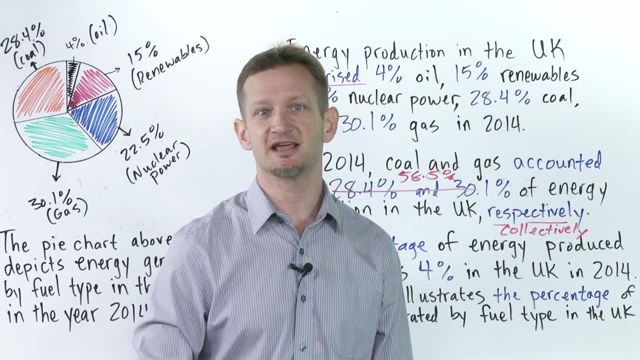 Alright, let's move on now a lot. So we talk about percent, right, five percent, twenty percent, twenty six point, four percent. That's important to be able to talk about that. But some students make the mistake of talking about percentage and they use it in the wrong, wrong context. 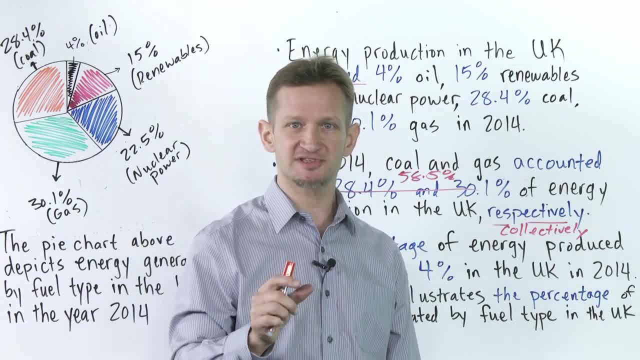 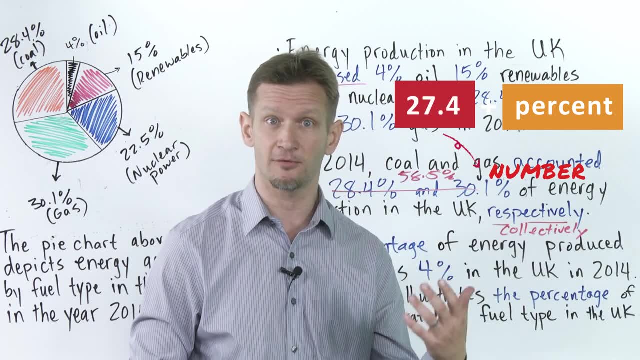 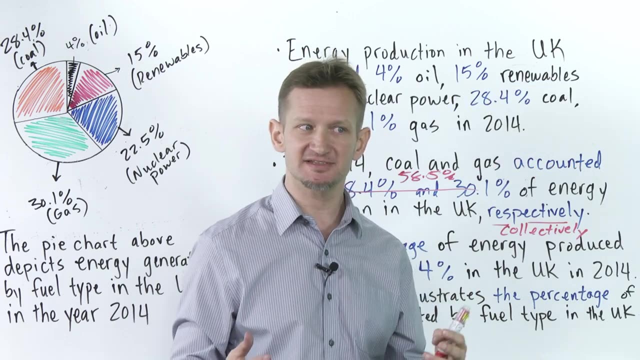 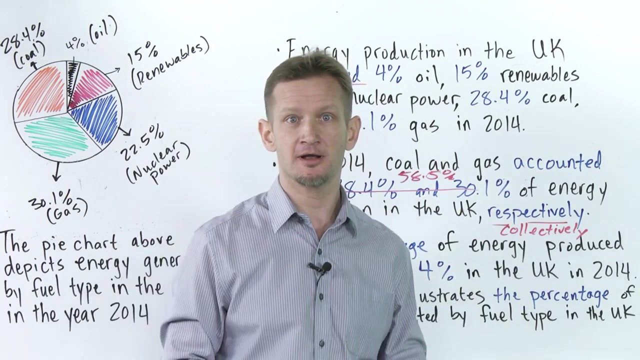 So here's a way to remember it: every time you say percent, It must have a number that comes before it: twenty five percent, twenty seven point four percent Percent must always be preceded by a number. now, percentage is how you can kind of talk about A portion of something that's separate from the number. Let me show you what I mean. 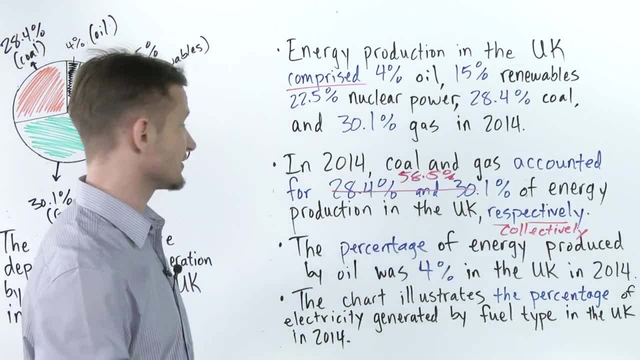 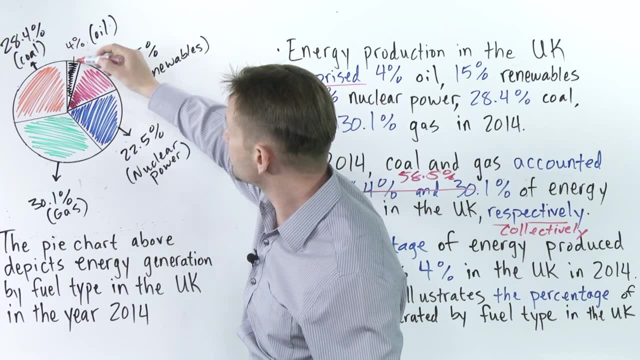 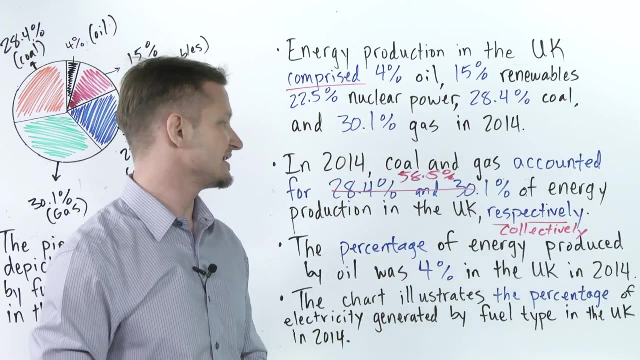 So the percentage of energy produced, right. so the graph, the chart, is all about energy produced and The percentage of energy produced by oil. okay, The percentage of energy produced by oil- I'm talking about that section, right. there Was four percent in the UK in 2014. 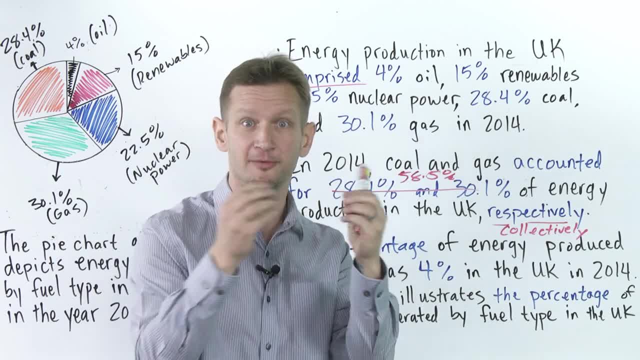 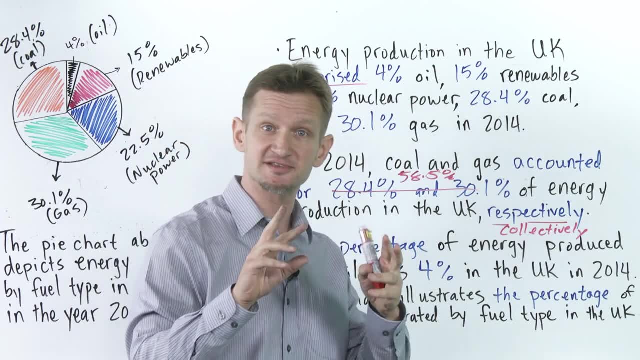 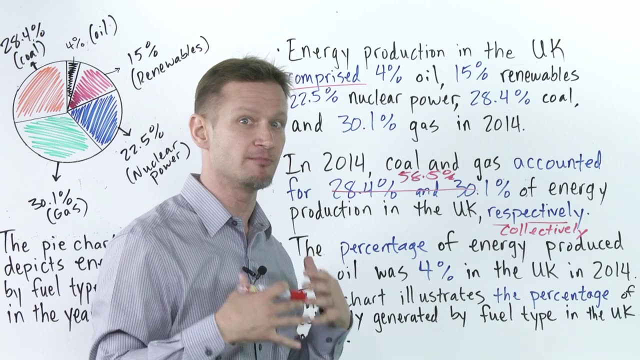 So that's just one way to kind of separate the number from percent, right, four percent becomes the percentage was four percent. It means the same thing, all right. so there's two ways to talk about percent there. But percentage you can use in a, in a, much in a different way. you can use it in in more, more ways than that. 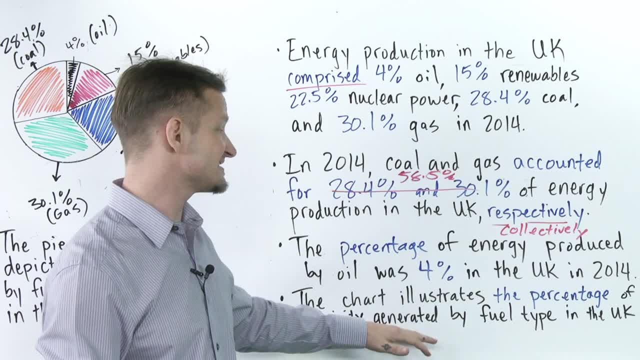 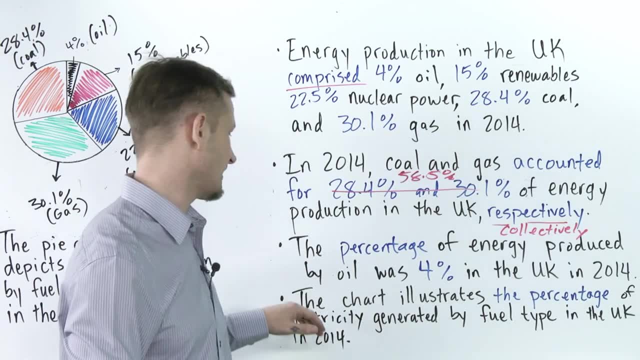 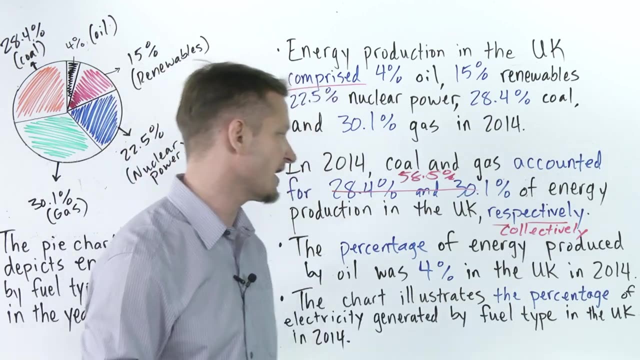 so let's look at a an example here. so here this sentence is going to talk about the entire chart. it's a way to describe the entire chart, you know, in a concise way. the chart illustrates the percentage of electricity generated by fuel type in the UK in 2014. so that's now we know exactly what the charts about. without 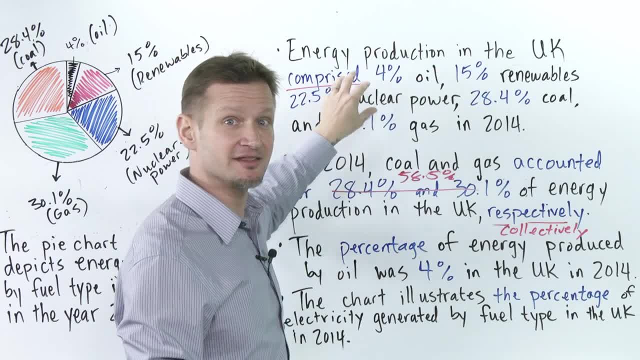 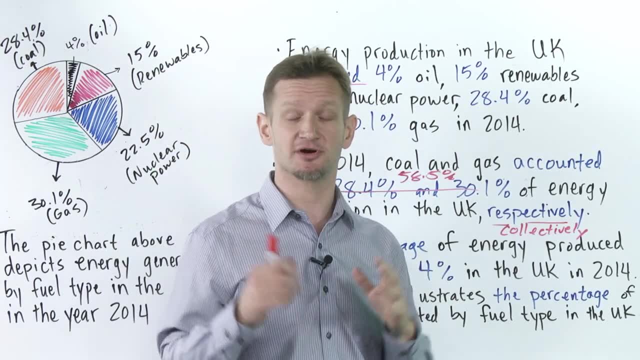 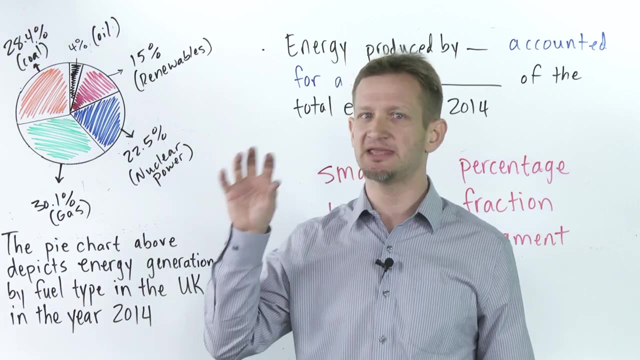 like going through and naming every the exact amount for every percent, as we did in this first example. so that's another way that you can use percent percentage. sorry, that's another way you can use percentage. okay, so now I want to talk, show you how to use percentage to talk about a piece of a whole, and it's 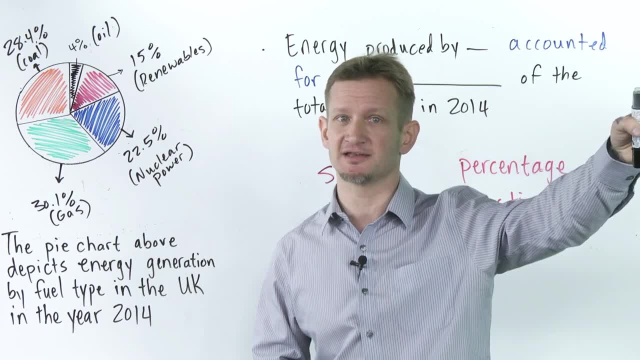 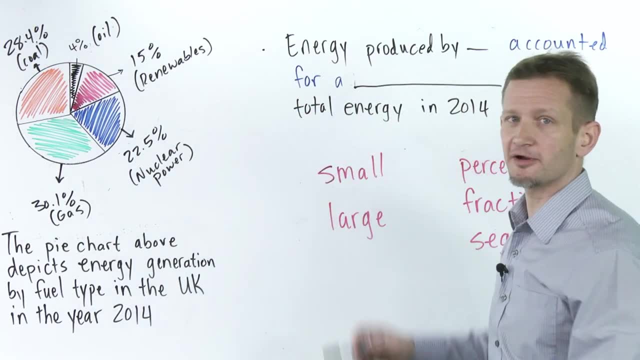 important, for you know that we're not talking about exact numbers. we're not talking about four percent. we're talking about small percentage or large percentage. let me show you what I mean. on the board here, I got a sentence with two blanks, and the first one, you add the piece of the whole so you can put. 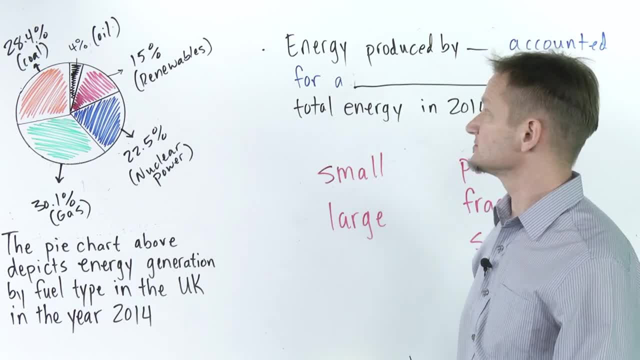 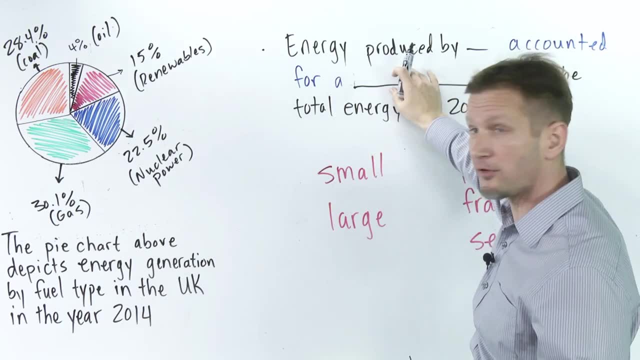 renewable energy and renewable energy and renewable energy and renewable energy. in here you can put nuclear power. so let's take oil, for example, as we already talked about. you could say energy produced by oil accounted for four percent of the total energy in 2014. we already talked about that. you can do. 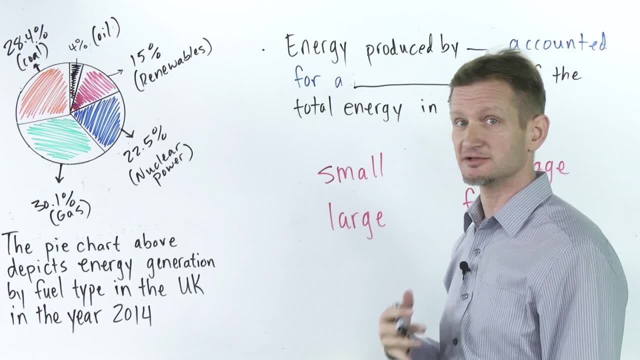 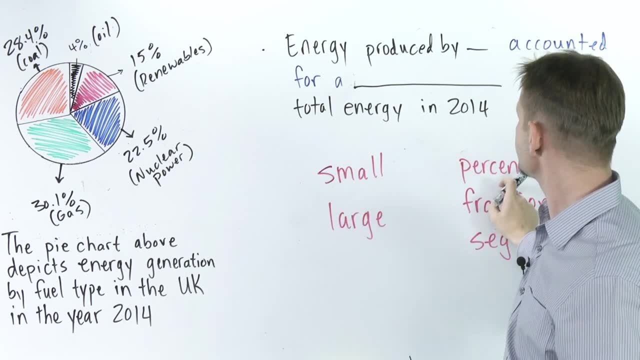 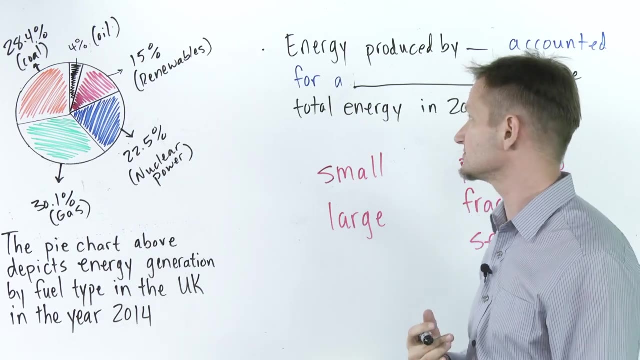 that. but if you wanted to add some diversity to how you're writing about this, then you can say: energy produced by oil accounted for a small percentage of the total energy in 2014. right, it's a way to vary how you're using these, these terms, how you're talking about this chart now. 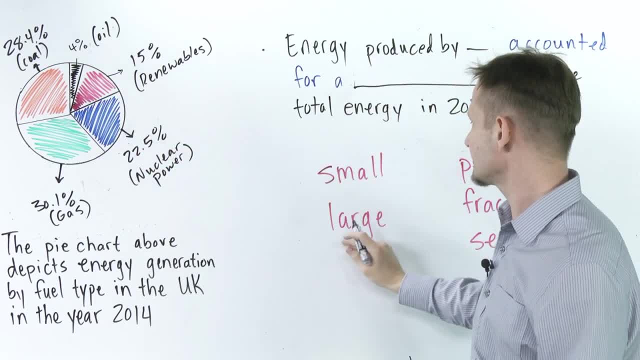 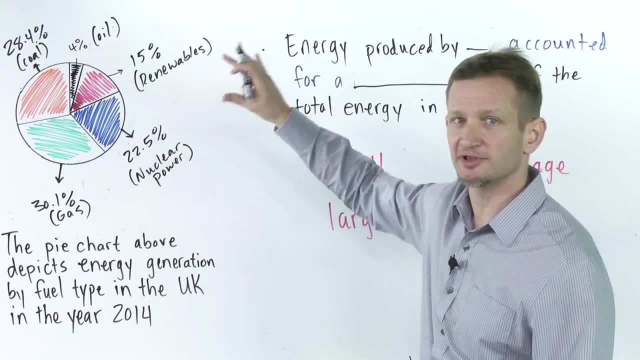 obviously, if it's coal, you're not going to say smallest percentage, you're going to say large percentage. so you have to, you have to think about what the small piece is in relation to the whole. is it small or is it big? now, also on top of: 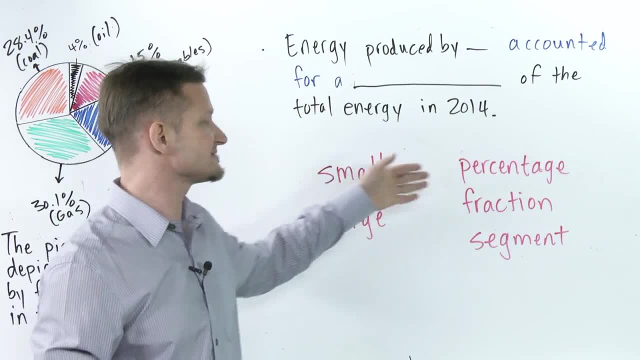 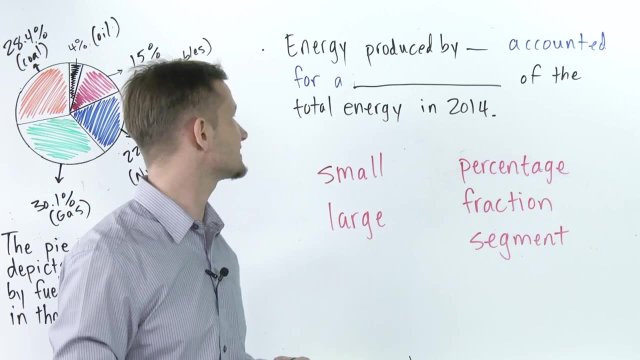 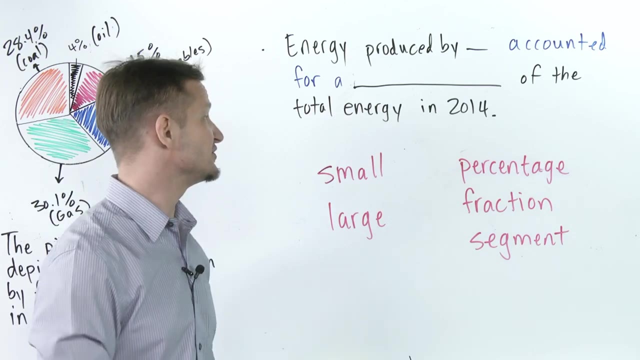 that you can say percentage, right, a small percentage, but you could also say a small fraction, you can also say a large segment. they mean the same thing in this case. they mean the same thing in this case. so that's another way that you can use percentage. now, if you wanted to do something else, you could even use: 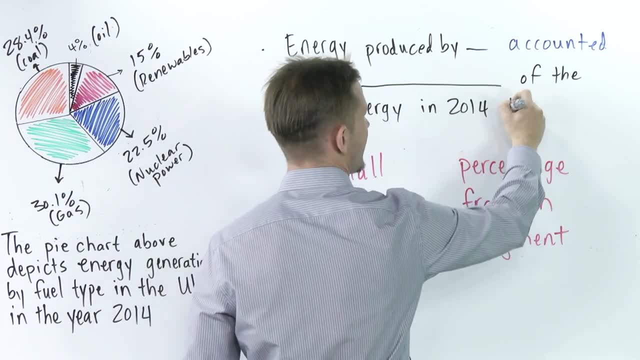 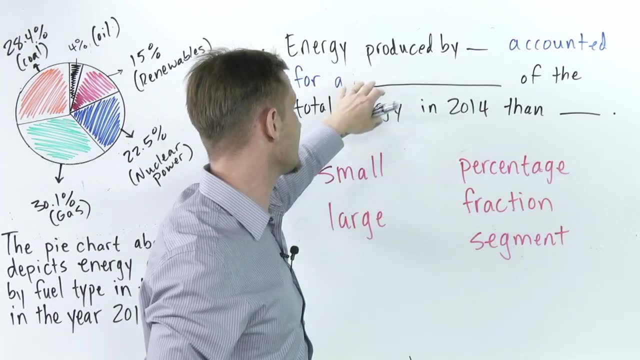 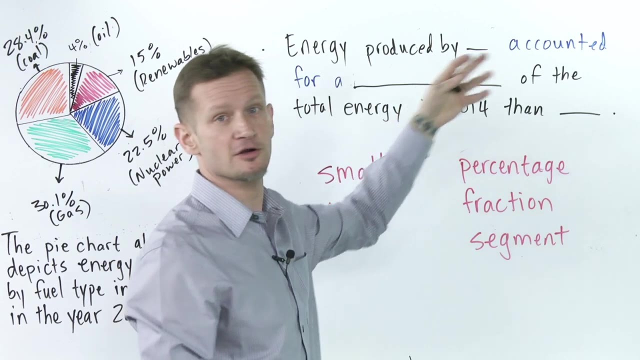 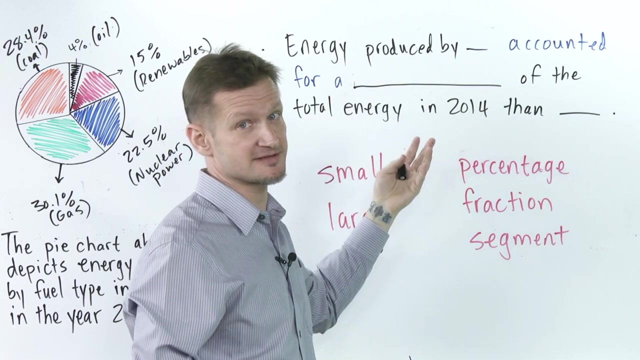 this to compare two things. you can add then, and you can put the second piece there: energy produced by oil accounted for a smaller percentage of the total energy in 2014 than coal, for example, so in that way, you can really take it up and make this sentence a comparative. 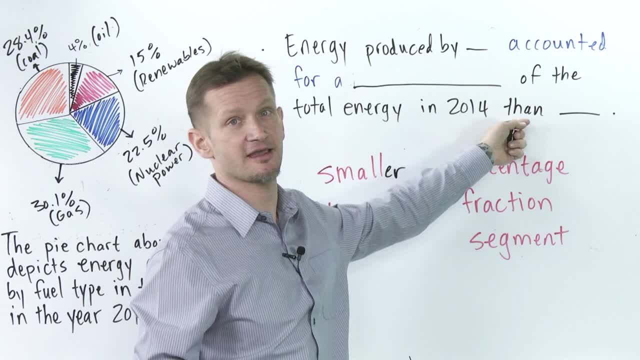 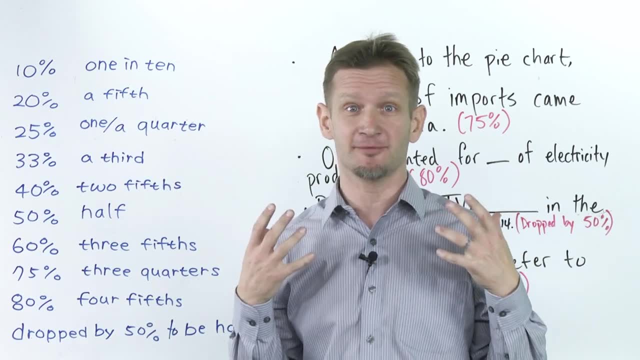 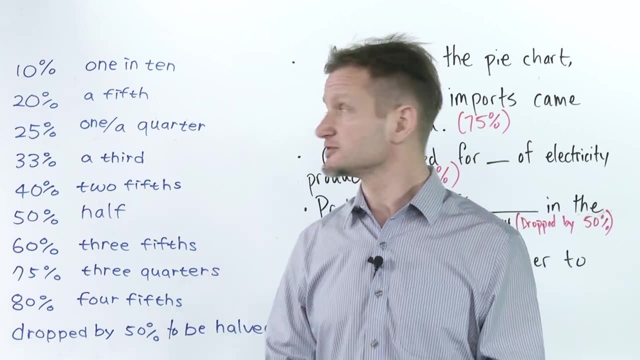 sentence by changing this to ER and adding than. and your second piece there. okay, if you haven't picked up the message that I'm trying to put down, it's that if you vary your vocabulary, you're gonna score higher, right? so now what I want to do is I want to show you a different way to talk about percentages. 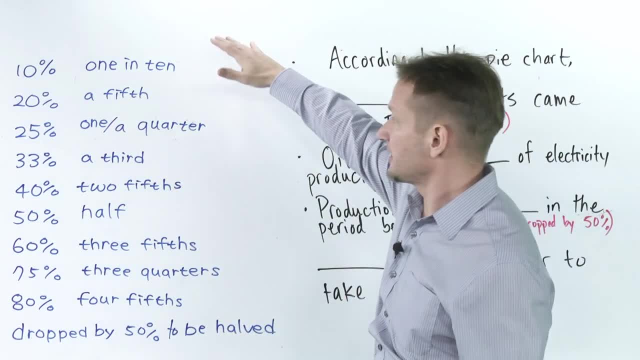 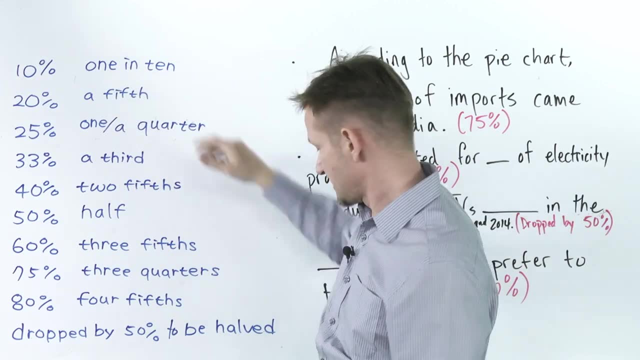 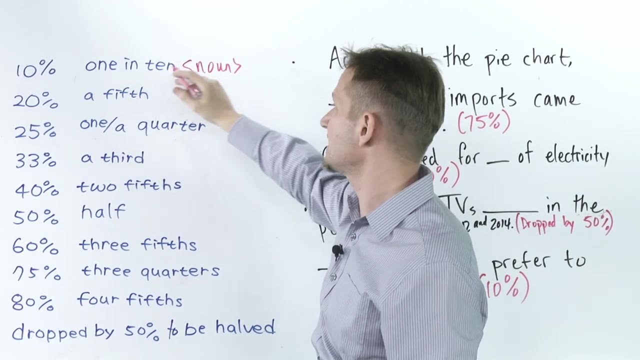 okay, so you here's, here's the percentage and here's what you would say. okay, so 10%, you can say 1 in 10 and then 1 in 10, and then you need to put a noun right here: 1 in 10 people, 1 in 10 schools, 1 in 10 countries. now, if it's 20%, you can say 2. 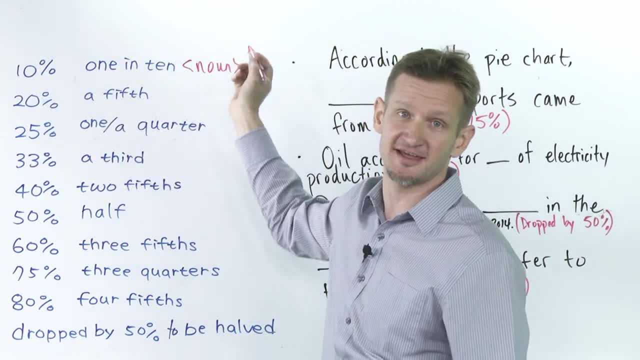 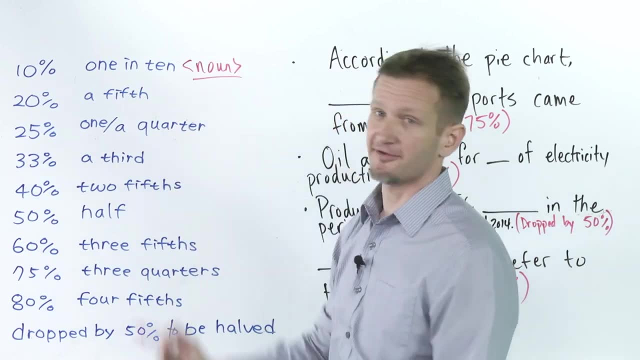 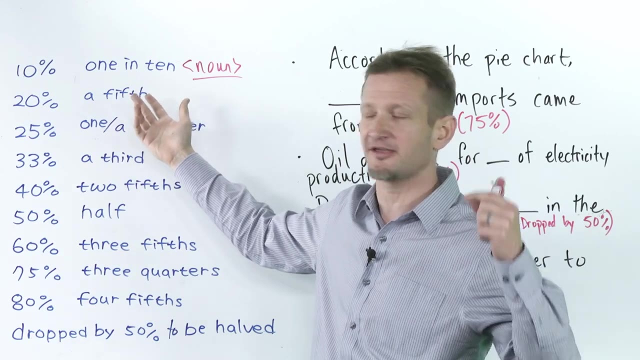 in 10. if it's 50%, you can say 5 in 10, if it's 70%, you can say 7 in 10. okay, just make sure you put a noun afterwards. and then moving on, so 20%. we also say a fifth, a fifth, make sure you get that a. 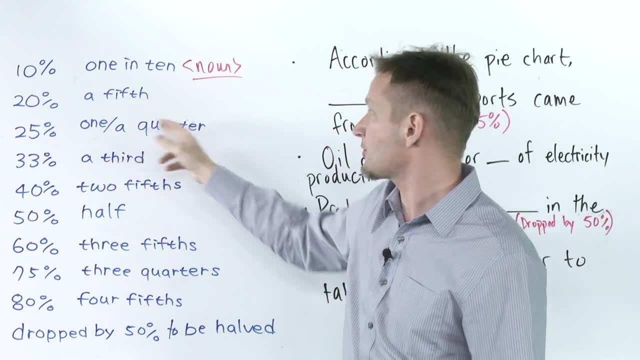 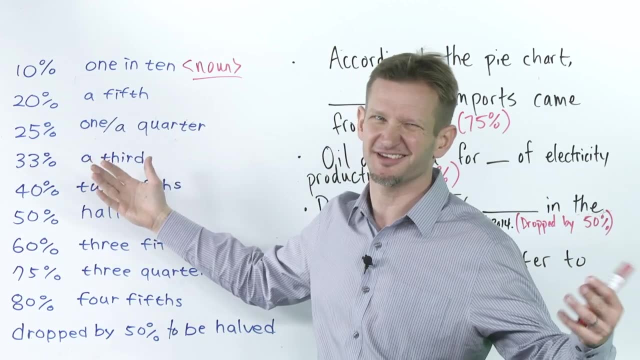 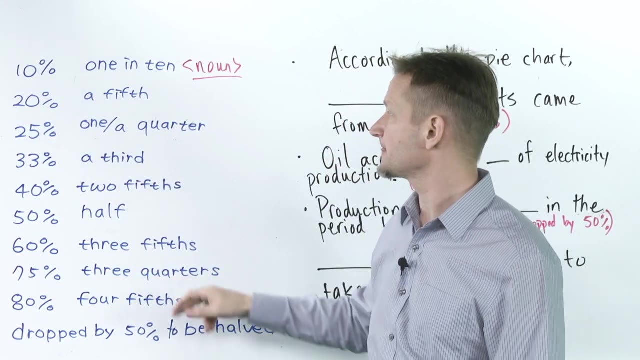 fifth, 25%. you can say a quarter or one quarter. so again, if it's 50%, you know we can say you could say two quarters. it'd be a little strange, so you'd really say half. if it's 75%, you're gonna say three quarters, 33%, that's a third, 40%, two. 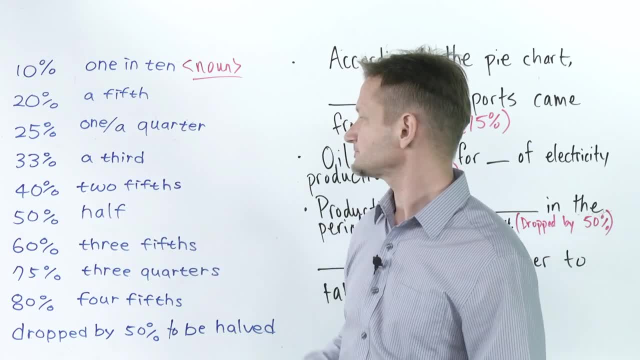 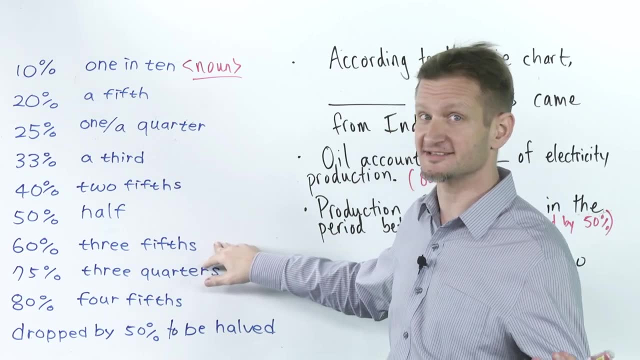 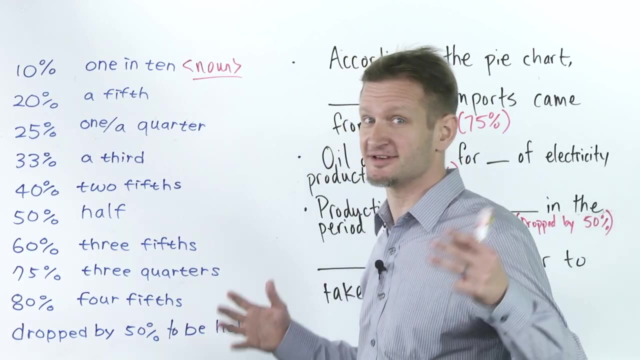 fifths. also, you can say four in ten, 50% is half, 60% is 3 fifths, or 6 and 10, both are okay. 80% is 4 fifths, 90% is 9 in 10. okay. so that's that's how you can use. you use words to talk about percentages. 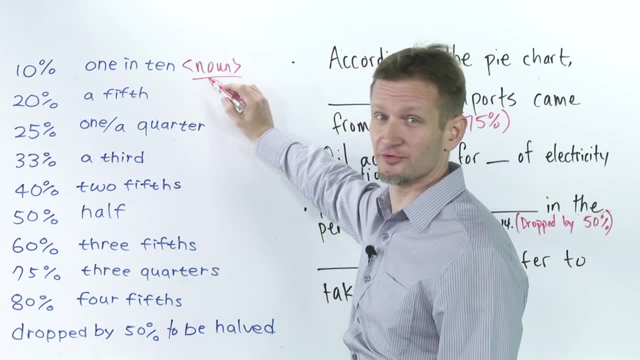 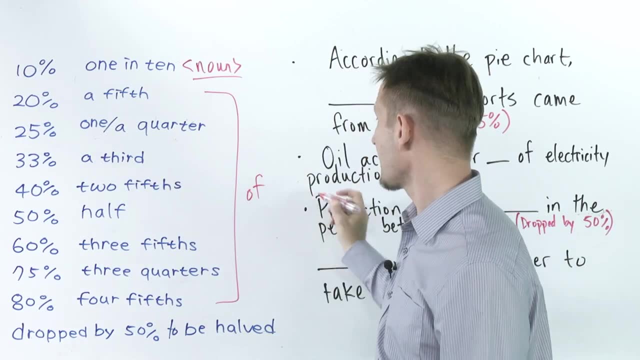 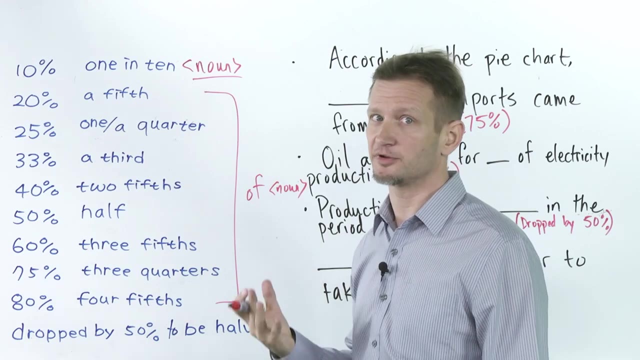 in a different way now here, 1 in 10 and then noun, right, so for the rest of these you gotta add of a third of, and then you put a noun. a third of noun, a third of energy production, a fifth of air pollution, for example. 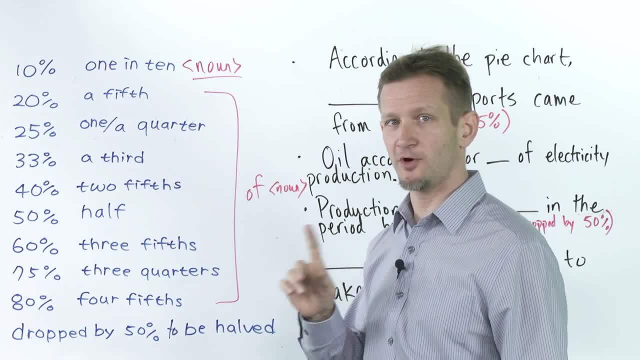 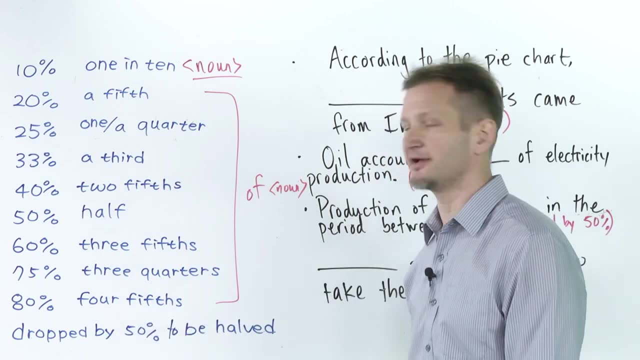 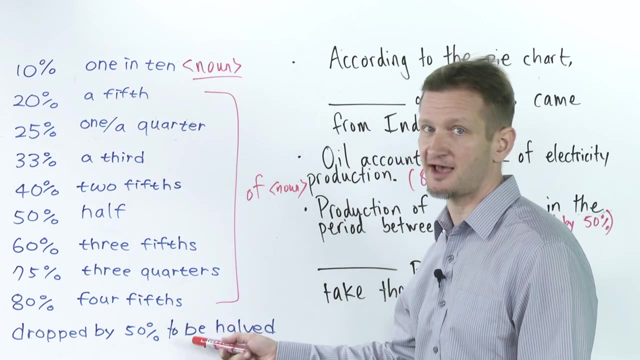 Make sure you put of and then a noun. So then I wanna give you one more really useful vocabulary, and that means to be halved. Now, when something's halved, it's dropped by 50%, It's cut in half. So you can say: right is halved, was halved. 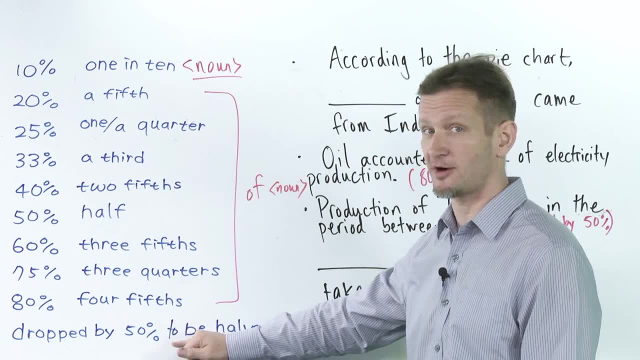 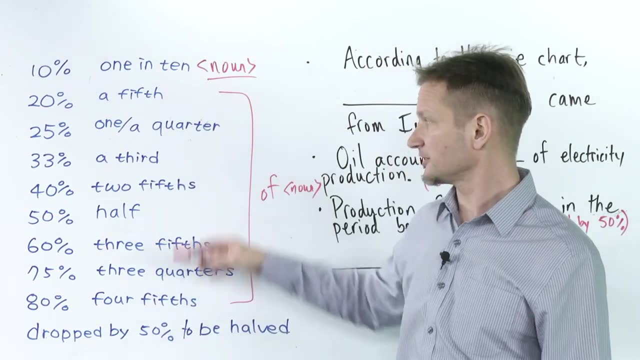 were halved are halved. You just conjugate to be into the proper form and then you add halved. Okay, now let's look at some examples. So we got our words here, our percentages in our words here. First example: according to the pie chart, 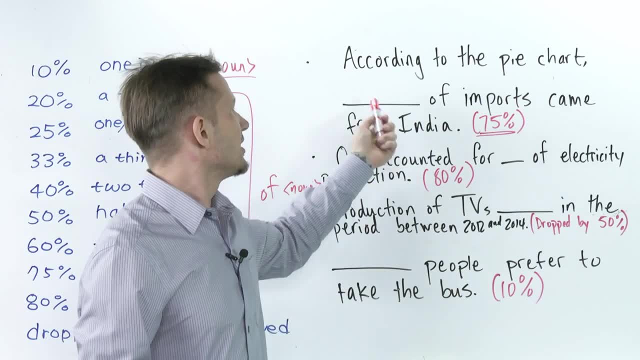 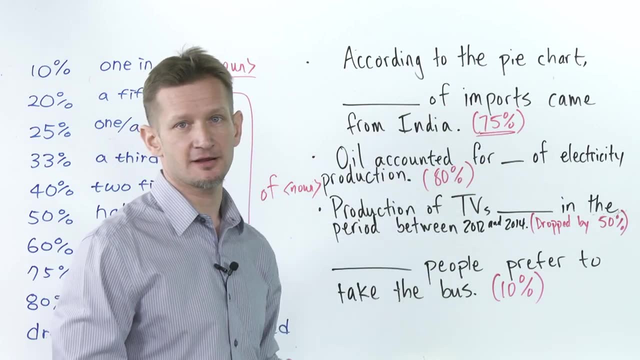 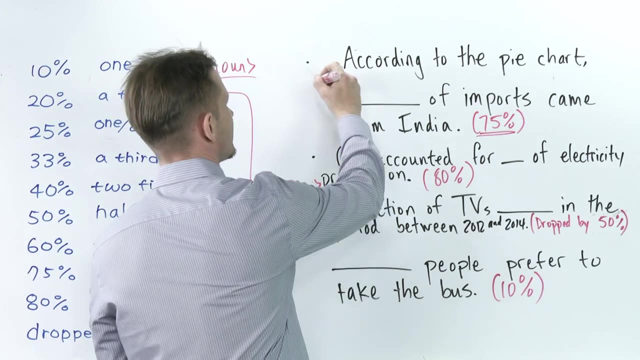 and we don't have a pie chart right, just an example sentence: how much, what percentage of imports came from India? Now we want a word that means 75%, right, And so 75% is 3 quarters. So we can say, according to the pie chart, 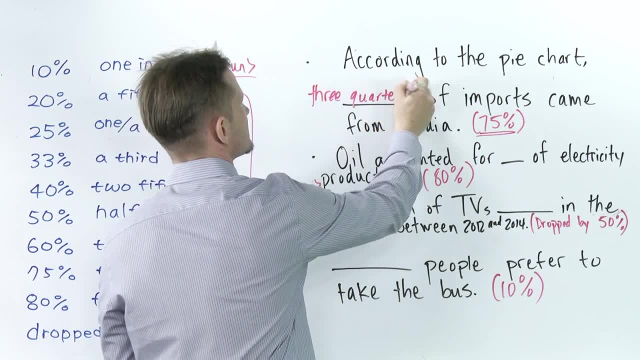 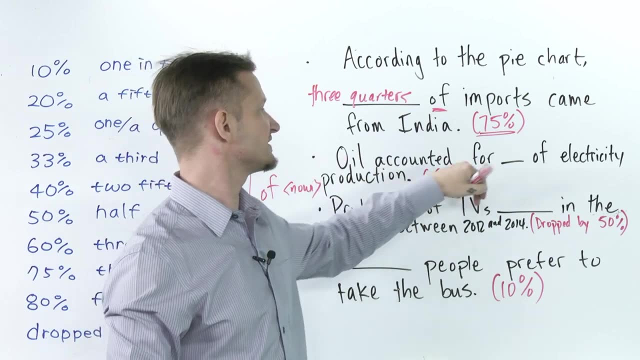 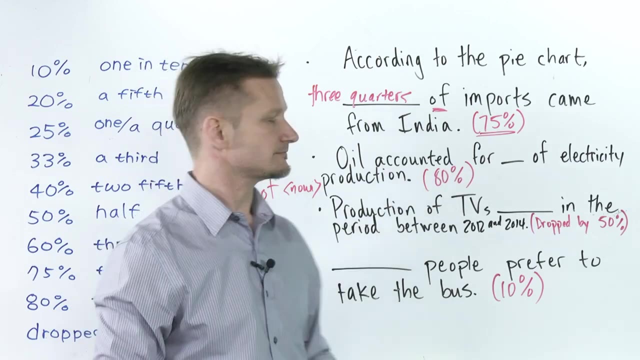 3 quarters of- and we got that of already there- of imports came from India. Next one, Oil, accounted for what percent of electricity production? So we want something that means 80%. So here can we say eight and 10?. 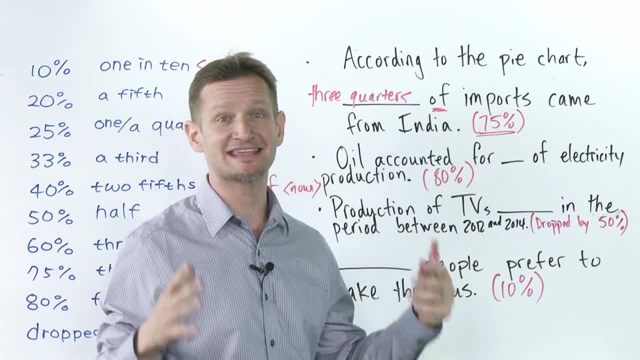 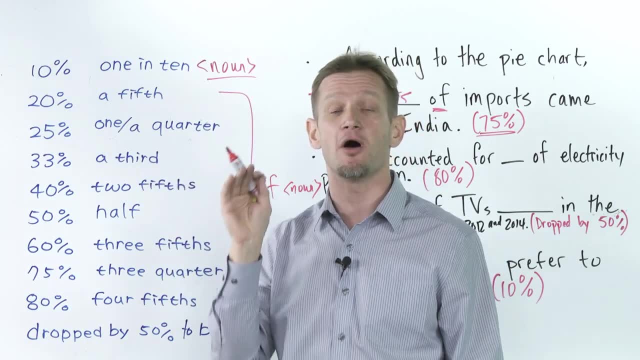 Can I say eight and 10 of electricity production? And you can't. And that's another thing about this. One in 10,, seven in 10, six in 10, you can only use with countable nouns. You can only use with countable nouns. 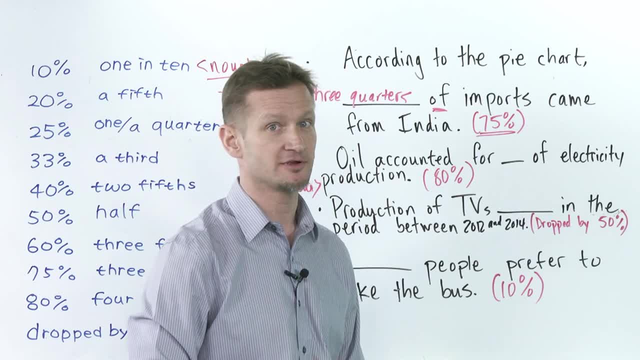 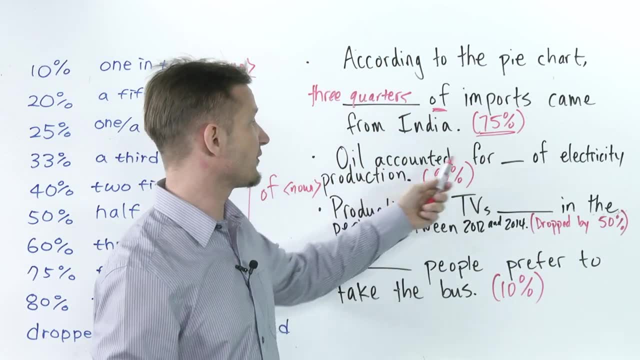 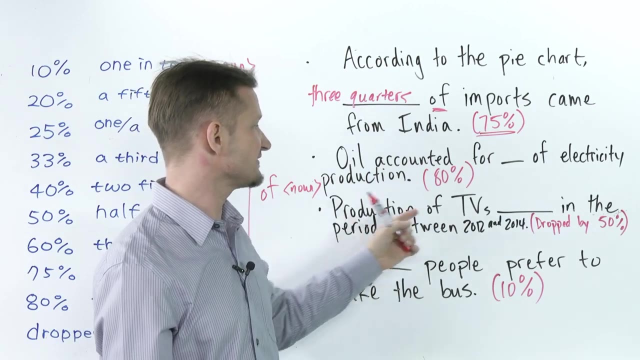 And electricity production is not countable, So we can't say eight and 10, but we can say four fifths. So oil accounted for four fifths of electricity production. Boom, All right. Production of TVs in the period between 2012 and 2014.. 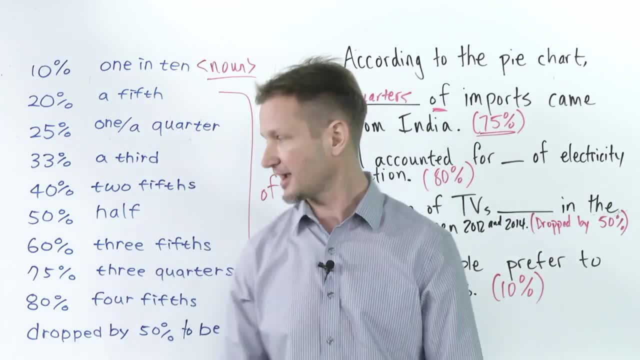 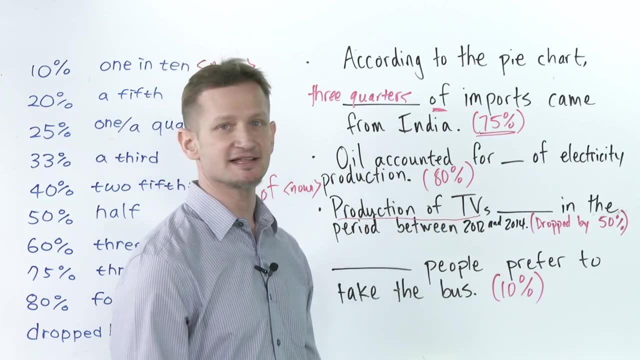 Now we want it dropped by 50%. Okay, To be halved, But we've got to conjugate the verb. So production of TVs. That's the subject of the sentence. So to be, we need to say that production, is it right? 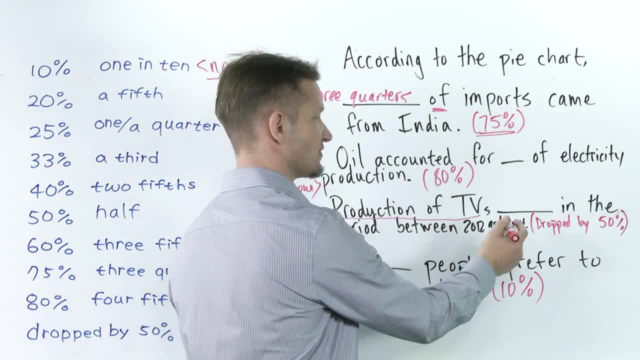 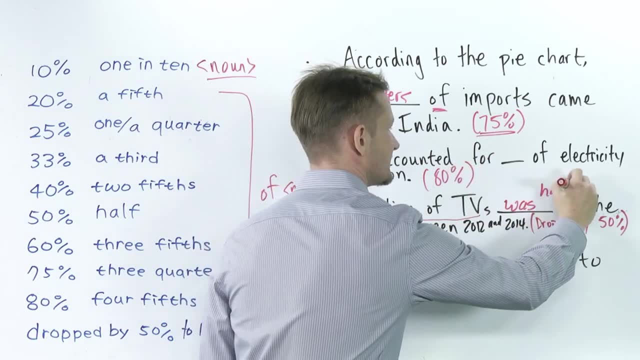 I, you, he, she it, we, they, It's it. So it we say was halved Was halved in the period between 2012 and 2014.. So for this one, when you're conjugating to be: 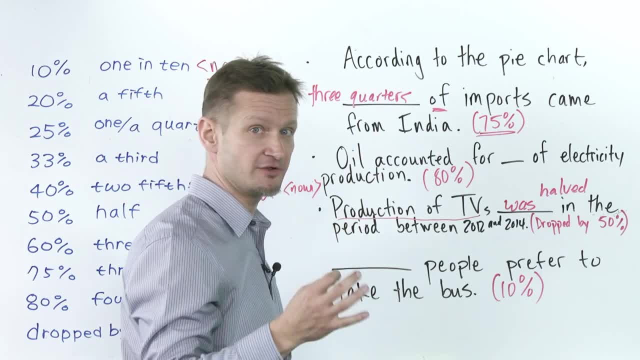 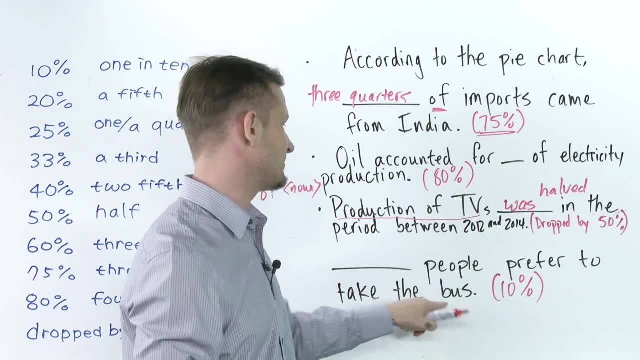 you gotta make sure you know what the subject is, And your subject's always I or you, he she it, we or they. It's always one of those. All right, so now people prefer to take the bus, So now, 10%, okay. 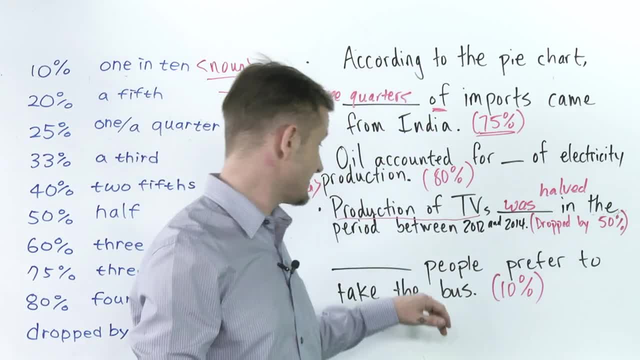 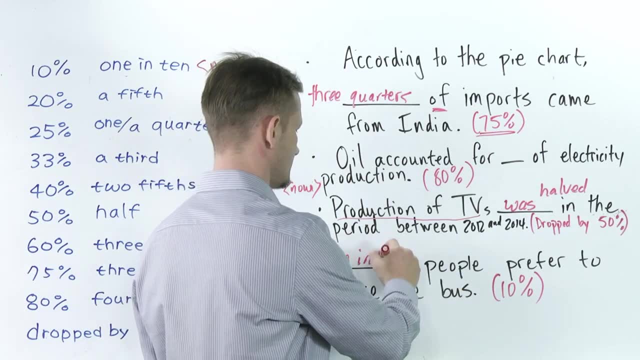 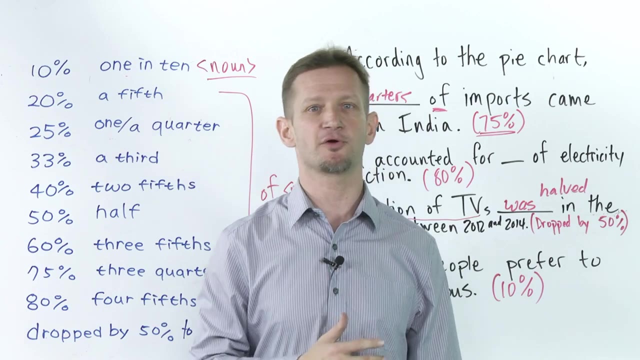 10%. one in 10, okay, Is people a countable noun? It is, So this is a safe place to use one in 10.. One in 10 people prefer to take the bus, And that's some example sentences of how you can use these words to vary your vocabulary. 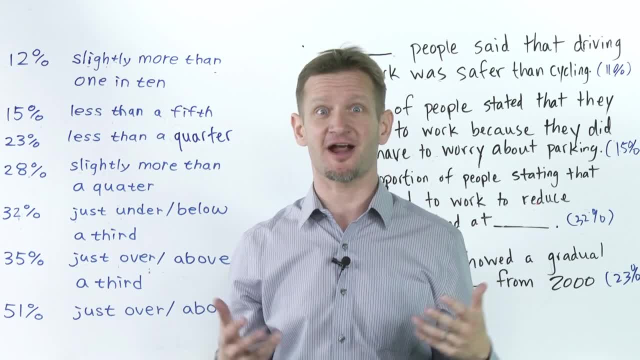 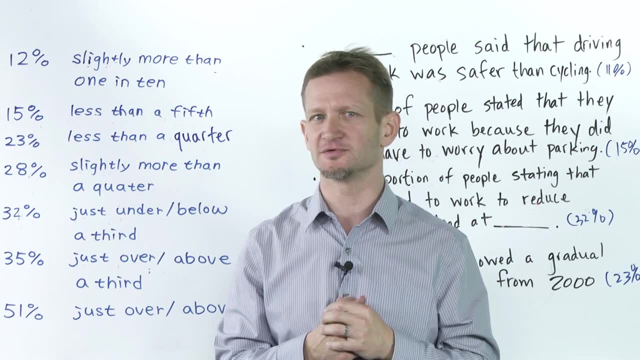 Okay, so we just talked about how to talk about these common fractions that we use in everyday speech. But what about if something's not quite those round numbers that we often use? Well, let me show you how to talk about those. So 12%, it's not one in 10.. 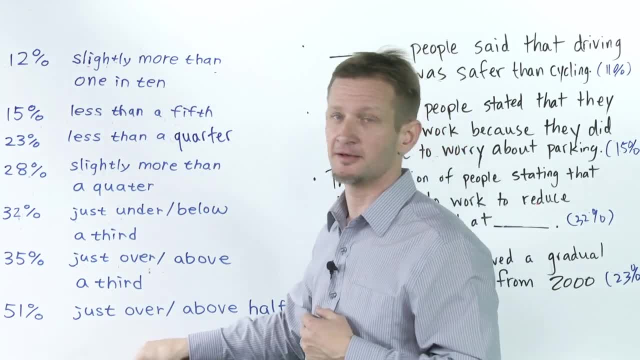 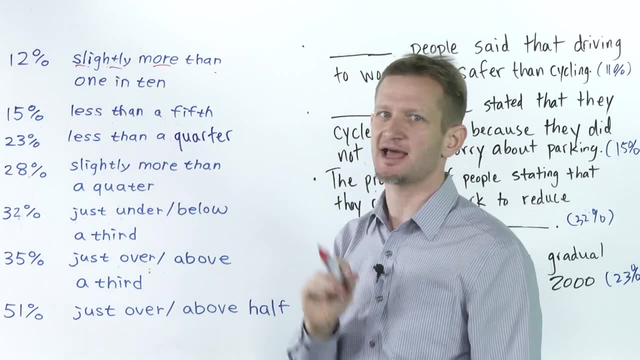 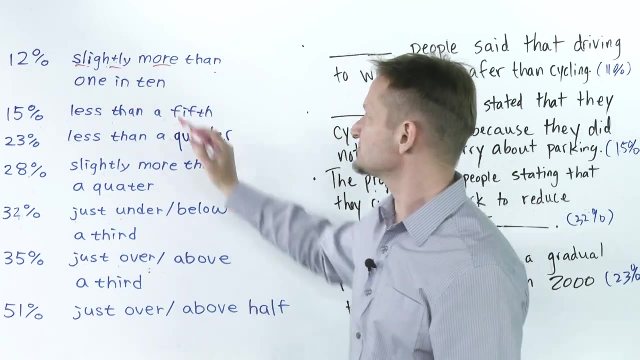 But it is slightly more than one in 10, right? So if you just add a modifier, slightly more than one in 10, that could be 12%. sure, It's not an exact number, and that's okay. You could also say slightly less than one in 10 if it's like 9%, all right. 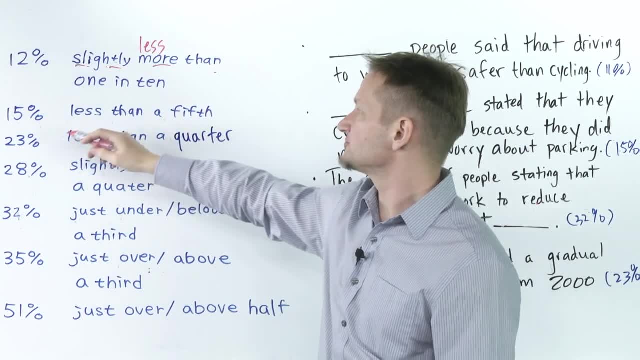 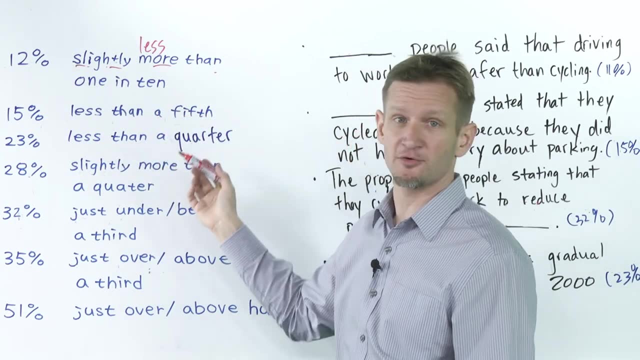 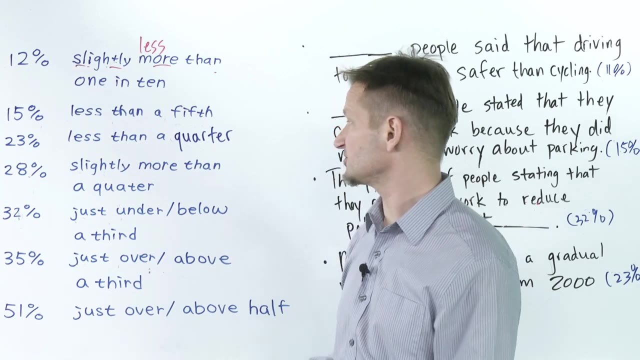 So you can change more to less, no problem. So for here, for 15%, that's not a fifth, but it is less than a fifth. 23%, it's not a quarter, but it's less than a quarter. So in the same way, like 28%, you can say slightly more than a quarter, or you can just say more. 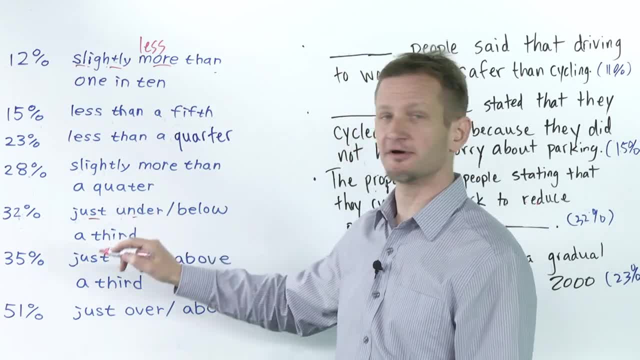 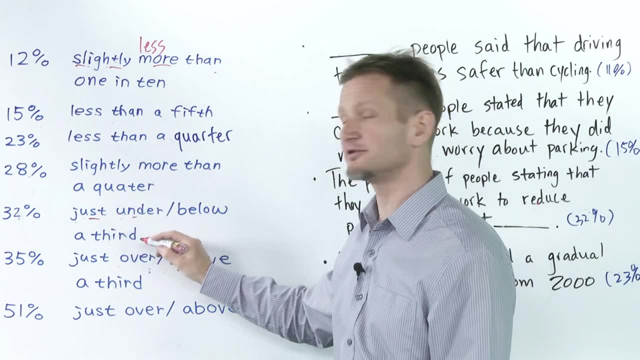 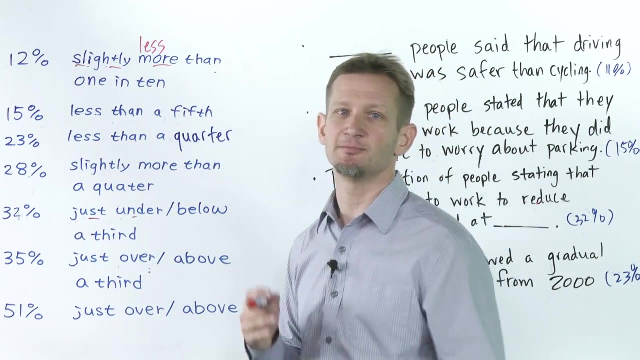 than a quarter, You can say just under a third, You can say just under a half or just over a half. So you can use these modifiers- just under, just below, just over, just above, slightly more, slightly less- to modify these very useful vocabulary. 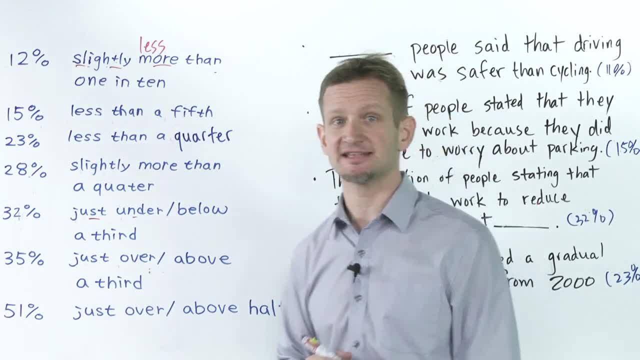 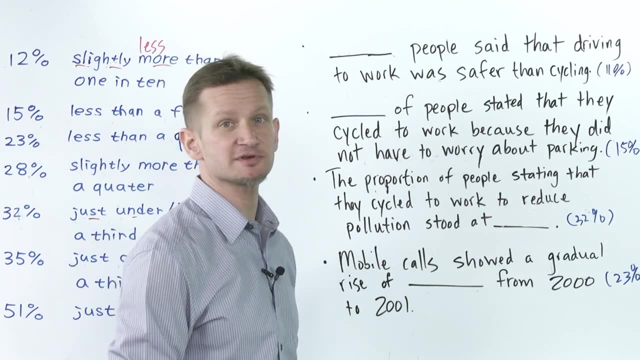 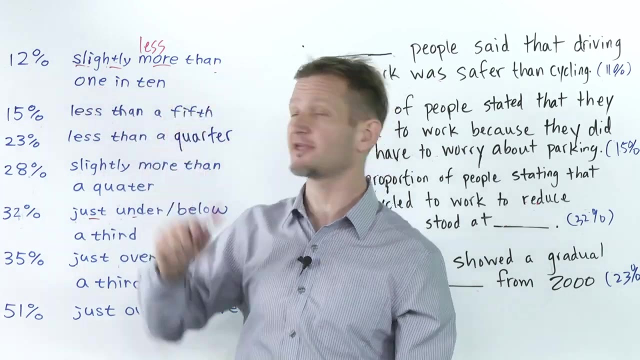 Okay. So now let's look at some examples, Some example sentences and how we can use them. So something of people said that driving to work was safer than cycling. Well, it's 11%. It's not one in 10, but it is slightly more than one in 10.. 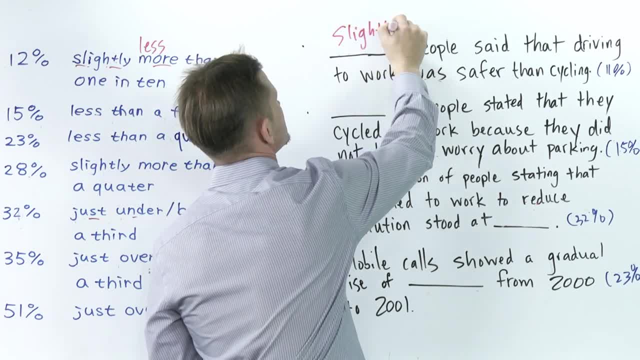 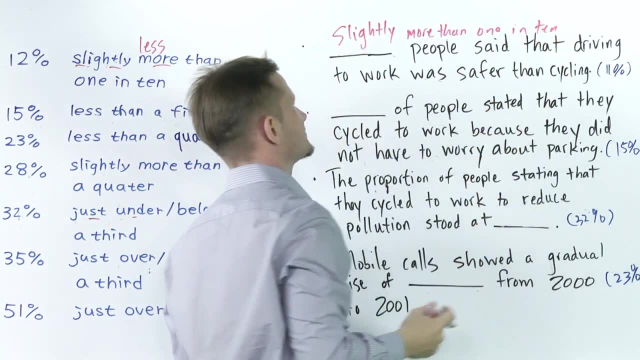 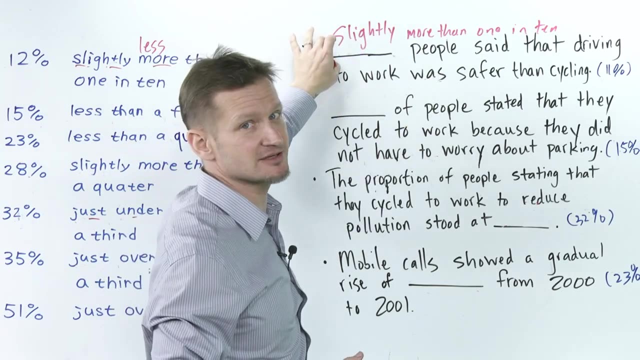 So we can put that in there Slightly. more than one in 10 people said that driving to work was safer than cycling. Great. Now you can say 11% of people. that's fine, but this is showing how well you can use the. 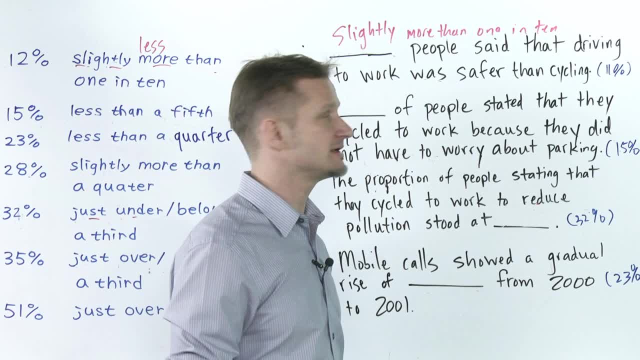 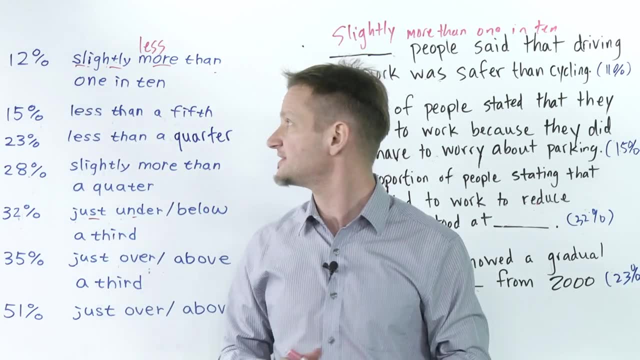 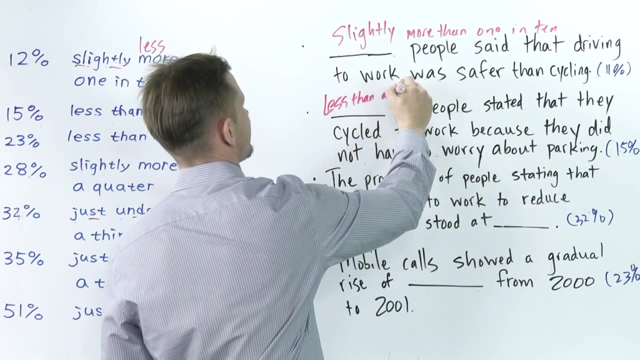 English language, You're using diversified vocabulary. That's important, Okay. So now we're looking for a number that means about 15%. Which one means about 15%? Well, we could say less than a fifth. So we can say less than a fifth. less than a fifth of people stated that they cycled. 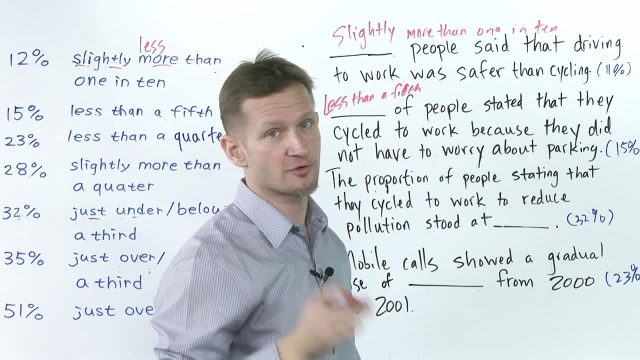 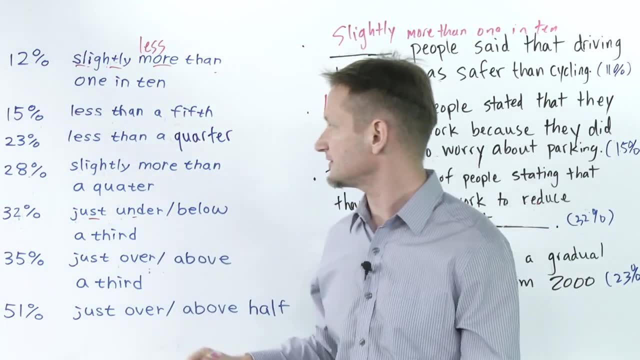 to work. Okay, They didn't have to worry about parking. Great sentence, All right. Moving on Number three, we're looking for something that means 32%. Okay, So we could just say just under a third or just below a third. 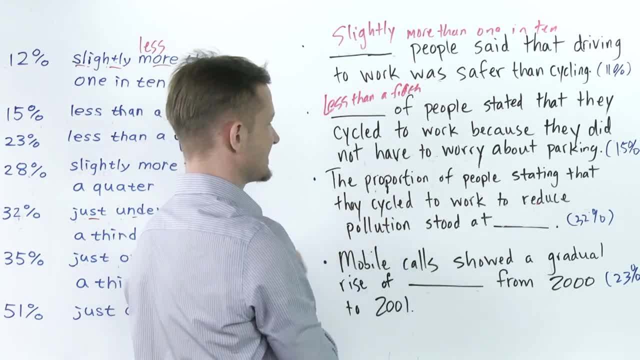 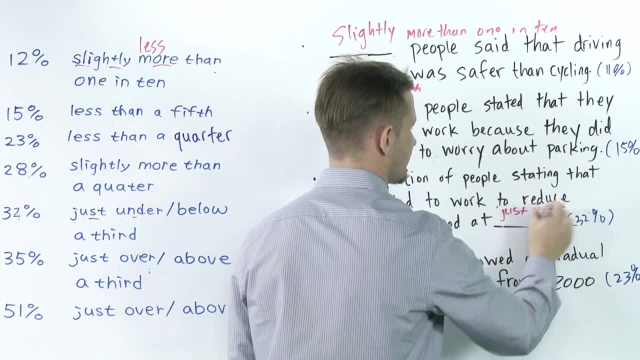 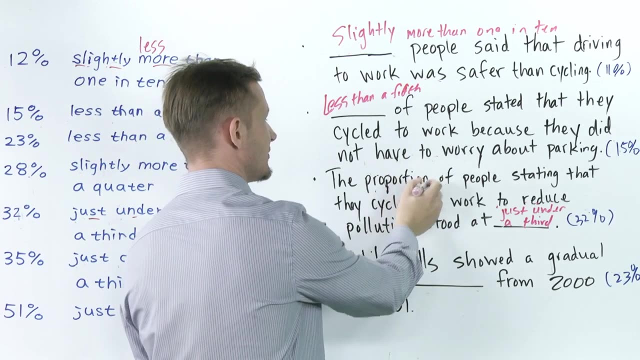 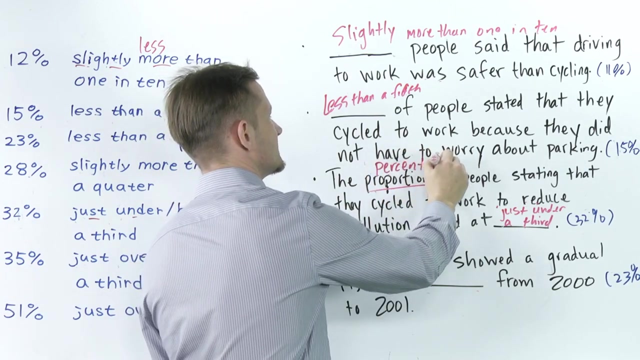 Both of those will work well. So we say: the proportion of people stating that they cycled to work to reduce pollution stood at just under a third. Okay, That's great. Now Let's talk a little bit about this sentence here We had. we say proportion and that's a great word, but you can also say percentage, the